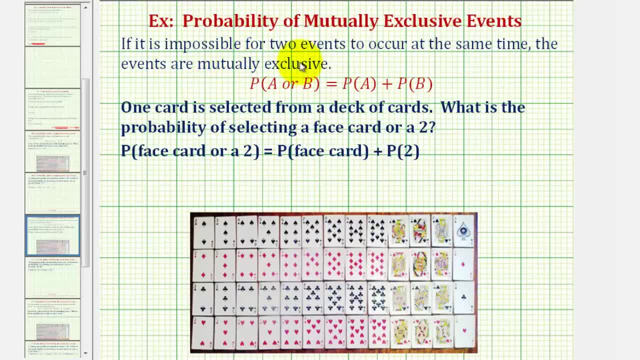 Welcome to two examples of determining probability of mutually exclusive events. If it is impossible for two events to occur at the same time, the events are called mutually exclusive. So if events A and B are mutually exclusive, then the probability of A or B is equal to the probability of A plus the probability of 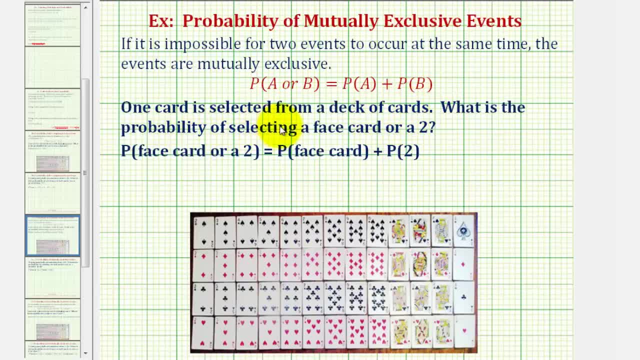 B. For our first example, one card is selected from a deck of cards. What is the probability of selecting a face card or a two? Since one card cannot be a face card and a two at the same time, these two events are mutually exclusive. 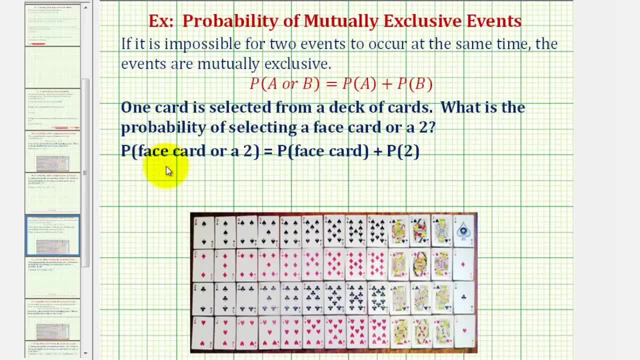 And therefore to find the probability of selecting one card and it being a face card or a two, we find the sum of the probability of a face card plus the probability of a two. A deck of cards is pictured here to assist us Notice there. 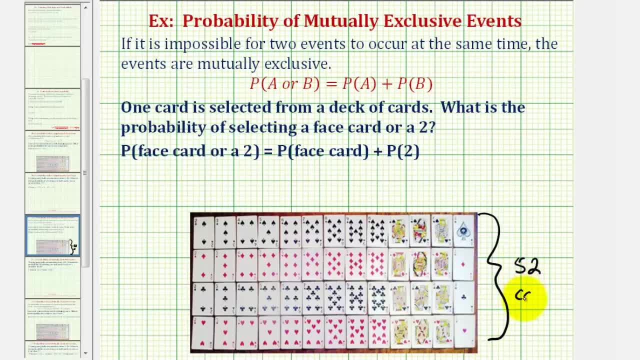 are fifty-two cards, Twelve of which are face cards. We have the jack, queen and king of each suit, And four of them are twos- Again one of each suit. So i think it's pretty easy to see that the probability of a face card or a two would be equal to twelve over. 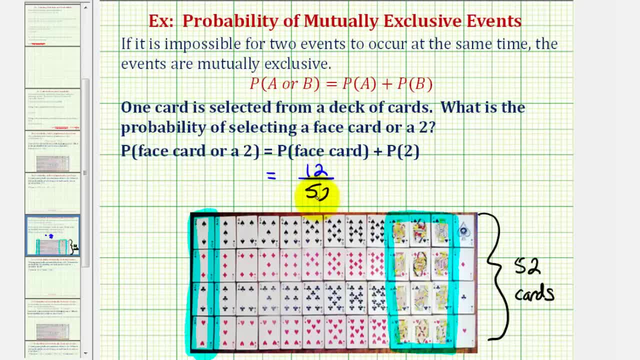 fifty-two the probability of selecting a face card, plus the probability of probability of a two, which would be four out of 52. So our sum here would be 16 out of 52.. And that should make sense because there are 16. 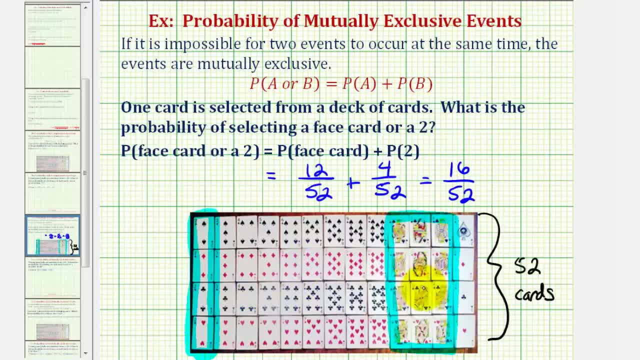 favorable ways of selecting a card, that is, a face card or a two out of a total of 52 cards. So this is our probability, but it does simplify. The greatest common factor of 16 and 52 is four. so if we divide both of these by four, 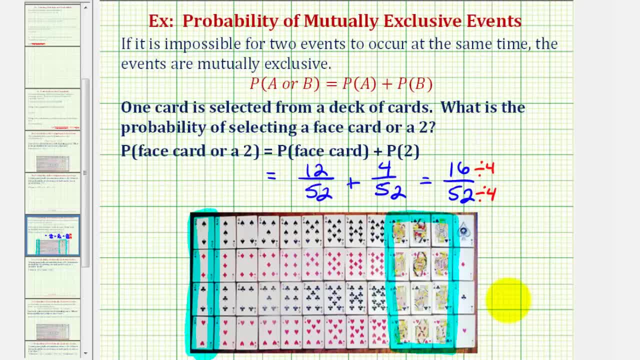 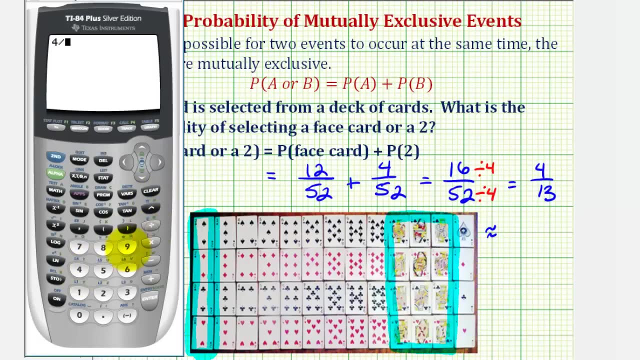 we would have the simplified fraction form of our probability, so this would be 4- 13ths. Let's also express this as a decimal and a percentage. So four divided by 13 will give us our decimal, So it's approximately 0.3077..